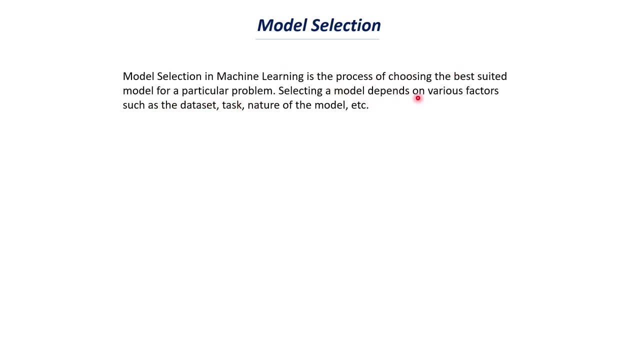 suited model for a particular problem. selecting a model depends on various factors, such as the data set task and nature of the model. okay, so this is about model selection. so we know that in machine learning we have lots of models. say, for example, we have a logistic regression model. 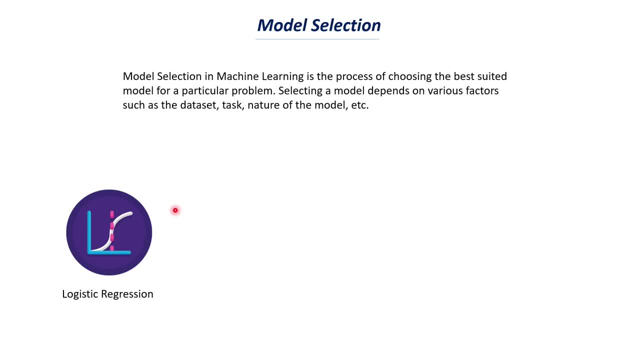 which is an example of supervised machine learning model, and then we have k-means clustering, which is an example of unsupervised learning model, and then we have a lot of different types of neural networks, which comes under deep learning. so similarly, we have other models, such as support. 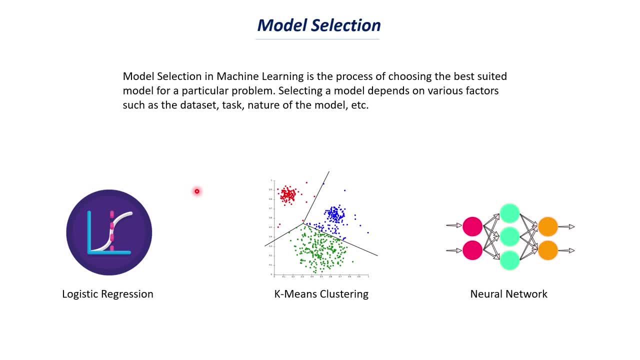 vector machine, hierarchical clustering, random forest, etc. and now we need to decide which model to use in which product or which, you know, project. so that question is answered by model selection. so we need to find the best model which is suited for a particular problem. okay, so this step is called as model selection and this depends on the data set that 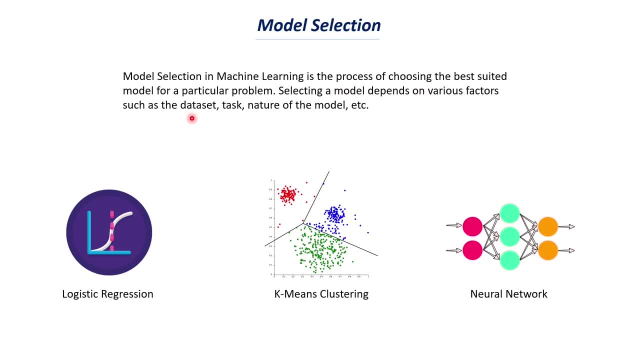 we have. okay, so based on the data set that we have, we may need to use different kinds of models and based on the task that we do. so task can be a classification task or a regression task. so classification task is nothing but classifying something, so it can be like predicting whether a person has a heart disease or not. okay, so in the, in this case, 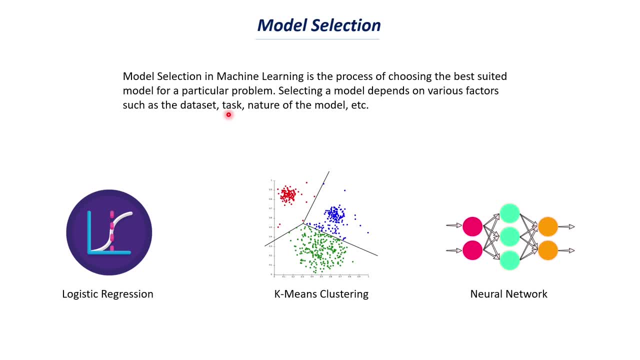 we are just predicting whether a person is having a heart disease or a person does not have heart disease. so we have two classes. so again, this is called as a classification problem. and then we have a regression problem where we try to find some value. so say, for example, we need to find 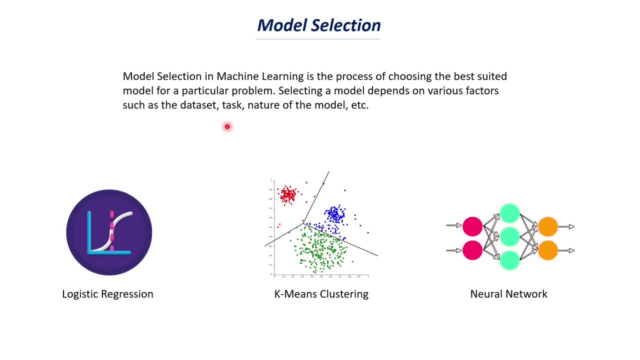 or we need to predict the house price. so price is nothing but a numerical value, right? so this type of problems is called as a regression problem. and then we have recommendation problems, etc. okay, so recommendation is there, forecasting is there, etc. so, depending on this task that we are, 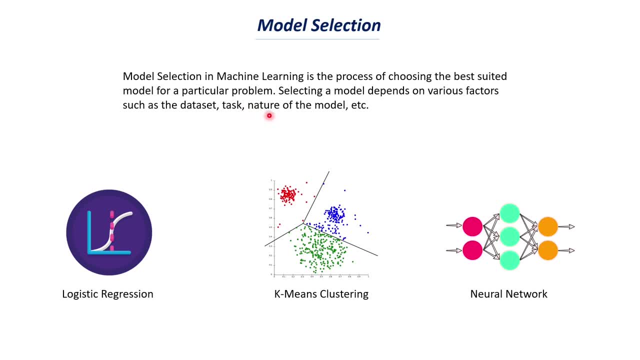 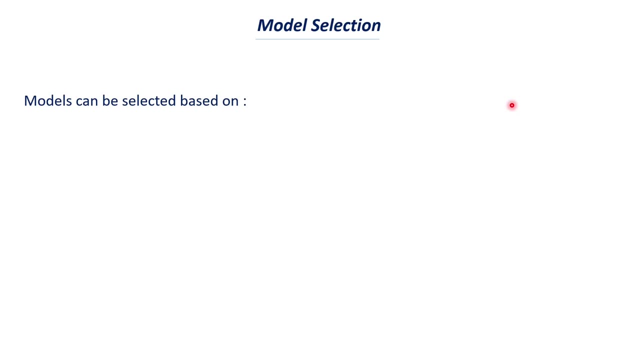 doing. the models that we select also changes, and also based on the nature of a particular model. so these are some factors on which we choose the models that is best suited for a problem. okay, so this is about model selection. now let's try to understand how we can choose the model based on. 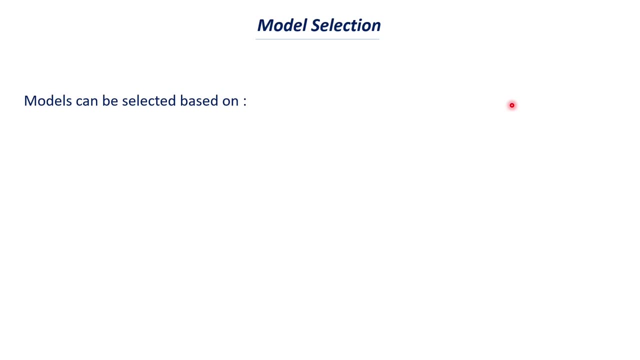 the data that we have and based on the task that we are doing. okay, so first let's discuss about the model. so if we have different kinds of data, we may need to choose specific models based on the data that we have. okay, so let's try to understand this. so, if we have a image or video data set in, 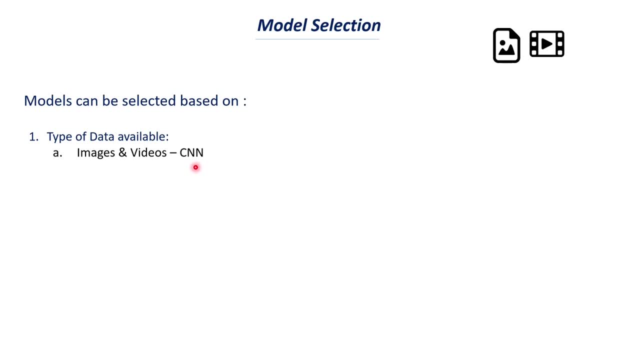 that case we use a cnn model. so cnn stands for convolutional neural network, so it is a deep learning model, so it is a neural network. okay, so because convolutional neural networks works better with images and video data set compared to other models, so in that case we use our cnn, so it can be. 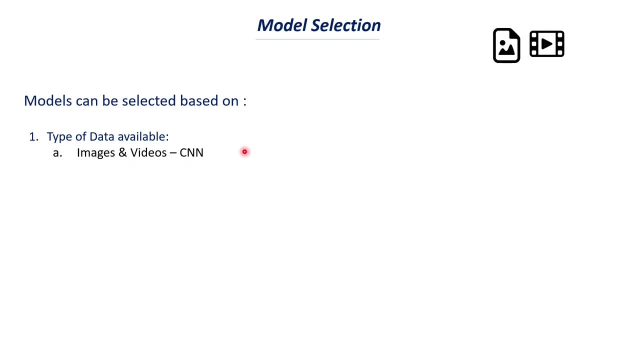 a face recognition problem or it can be a clicking other image represents a cat or dog and such kind of things. so in that cases we use a cnn and when it comes to text data or speech data we use rnn, and rnn stands for recurrent neural networks and these two are deep learning models. so these kind of problems that involves a speech, 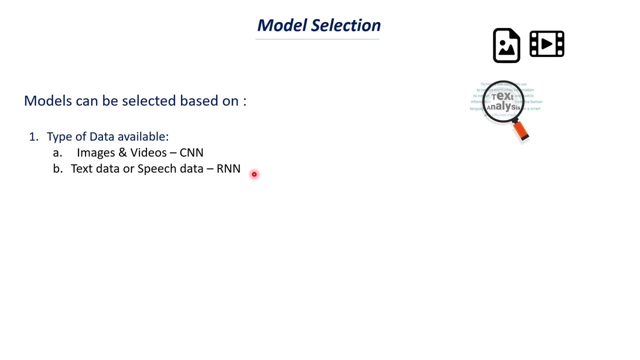 data and text data is also called as time series problems. so, and in that cases we use rnn, because rnn works better. in those cases, and when we have some simple numerical data, we use simple machine learning models, such as support vector machine models. we can also use logistic regression. 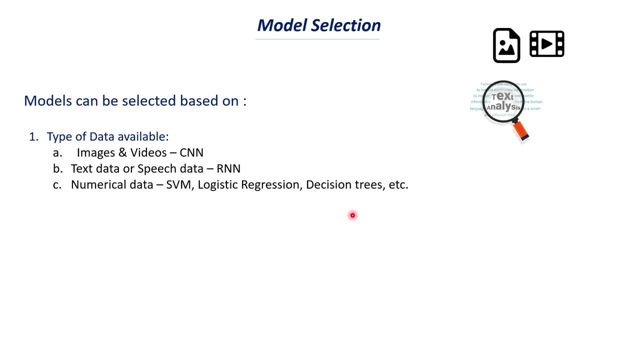 decision trees, etc. okay, so this is a thumb rule that we generally have in machine learning. so in the case of image and videos, we go with deep learning, where we use cnn, uh models, and when it comes to text data or speech data, we use recurrent neural networks, also known as rnn. and for simple, 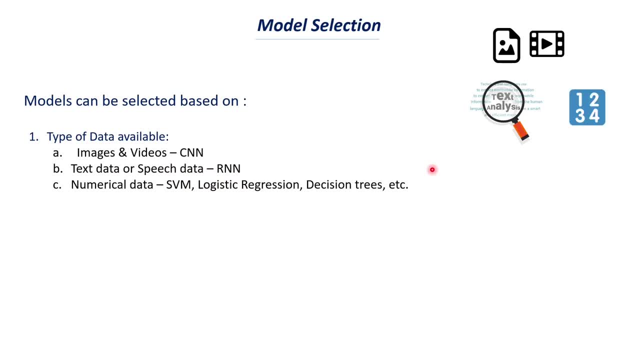 numerical problems, we can use these kind of models. okay, so now let's discuss how to choose the models based on the task that we do. so, when it comes to classification tasks, use a support vector machine model or a logistic regression or a decision tree. okay, so classification. 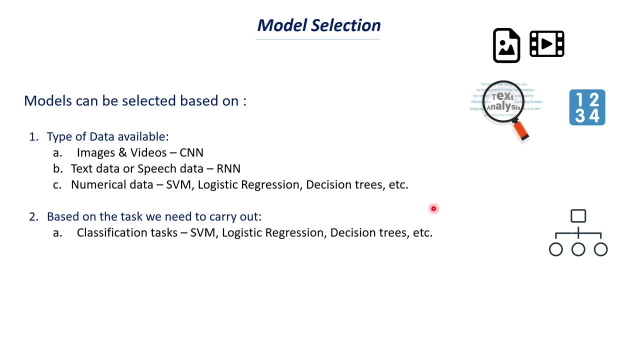 as i have said before, we need to classify something. so it can be like, as i have told you before, it can be like predicting whether a person has diabetes or not. in this we are just classifying with two output variables. okay, so one is the person has diabetes and the second outcome is: 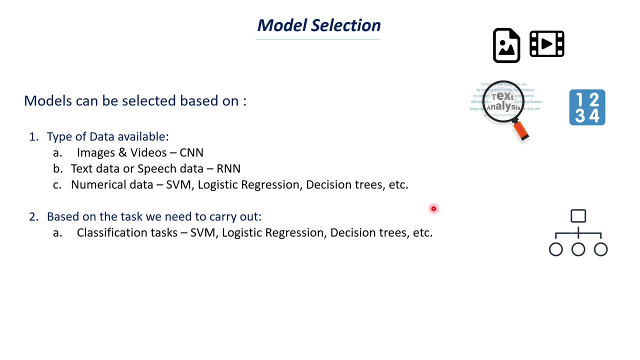 the person does not have diabetes. so this is an example of a classification task. and then we have regression, where we try to find some value. so it is like predicting a car price based on its parameters- few parameters. so this is an example of a regression task where we find some numerical. 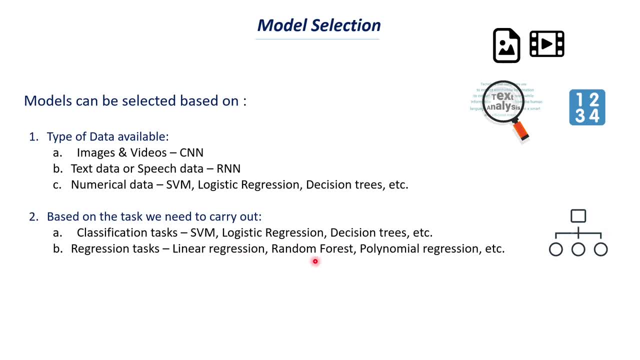 value, and in that cases we may use a linear regression, random forest regression, polynomial regression, etc. okay, and one main thing to note here is that few models can be used for classification and regression as well. okay, for example, support vector machine can be used for both classification and regression. so you need to take note. 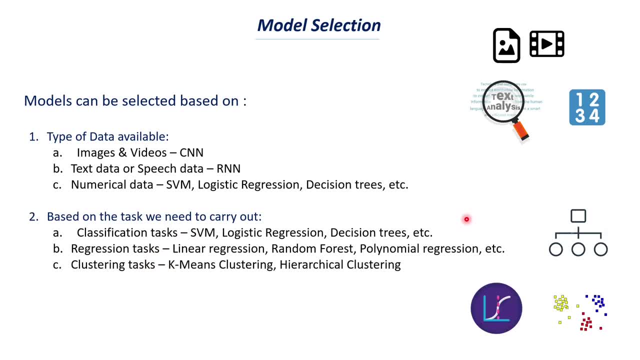 of that. and then we have clustering test. okay, clustering is like we try to group the data set based on the similarities. so in our youtube channel we have did a project on customer segmentation we where we tried to group customers based on their spending pattern. so this is an 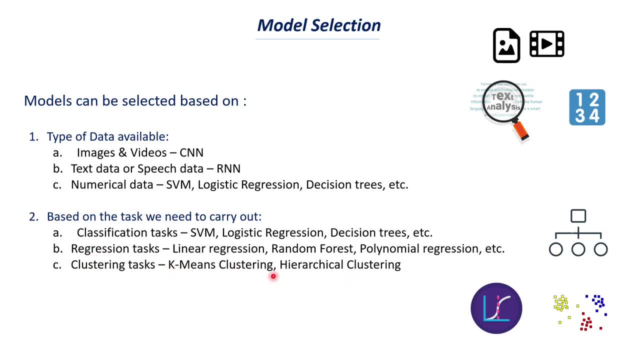 example of a clustering task, and in that cases we can use k-means clustering model or hierarchical clustering model. okay, so this is a- you know, a gentle introduction of model selection. so these are the different types of models you can use, based on the type of data. 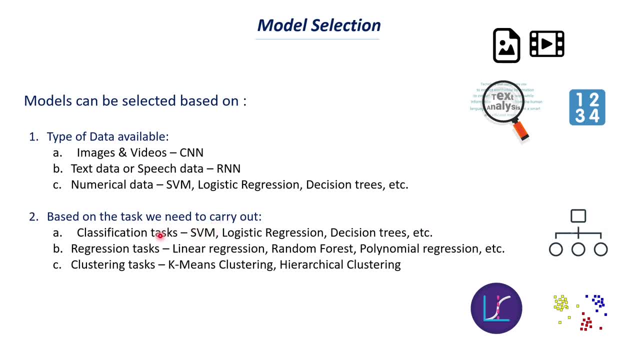 that we have and based on the task that we do. okay, now you may ask a question that in classification we may use a support vector machine or logistic regression or decision trees, but how to choose the best model for a classification test? you may ask that question. okay, so it depends on various 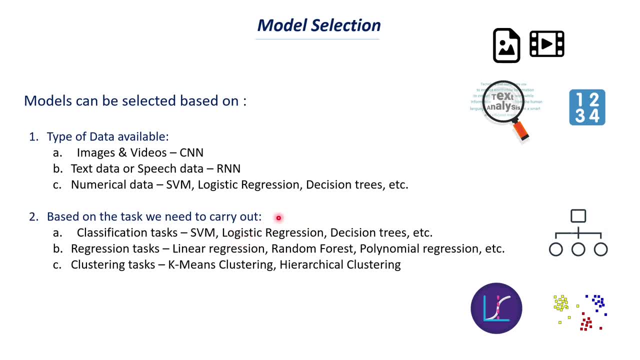 parameters as well. say, for example, we use logistic regression when we have binary classification. binary classification is when we have only two classes. okay, so in that case we use a logistic regression. and when it comes to svm, there are also a few things related to it, so we use a support. 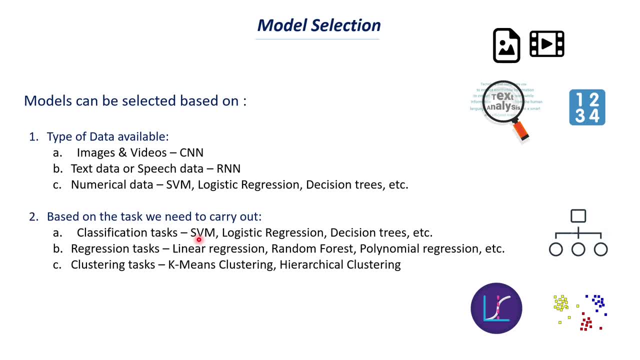 vector machine model when the data is, when the data set is very small and there are no outliers in the data. when there are a lot of outliers in the data, support vector machine cannot work well. and it does not also work well when the data set is too large because the processing time is more. 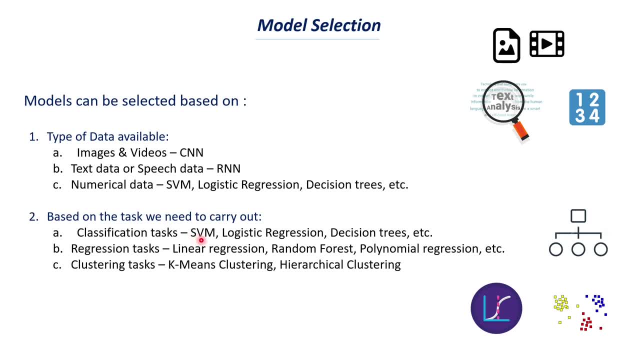 with a support vector machine, so it is very sensitive to noises or outliers. so, like this, there are a lot of parameters that we need to consider before choosing a particular model, so in the upcoming videos we will discuss about all of these individual models, and so in that, 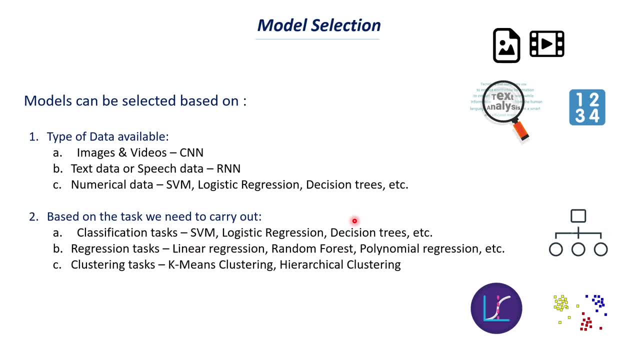 videos i will be explaining you the pros and cons. so, based on these pros and cons, we need to choose the proper model which is best suited for a particular problem. okay, so i cannot explain you all those things in this video, so we need to understand about all these models before. 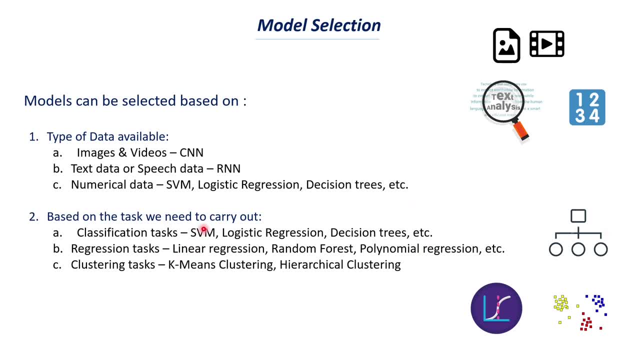 uh, going into that part, okay, so just uh, keep in mind that there are few parameters about models that we need to take care of before selecting the model. okay so, but this is the general rule. so for image and videos, we use cnn. for text data and speech data, we generally use rnn. 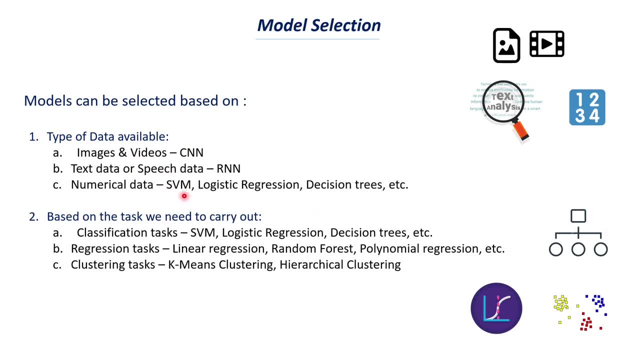 and for a simple numerical data we can go with machine learning models like svm, logistic regression, decision trees etc. and for classification we kind of use these models and for regression we use some regression models and for clustering use k-means clustering and hierarchical clustering. okay, so this is all about model selection. now there is another topic which we need. 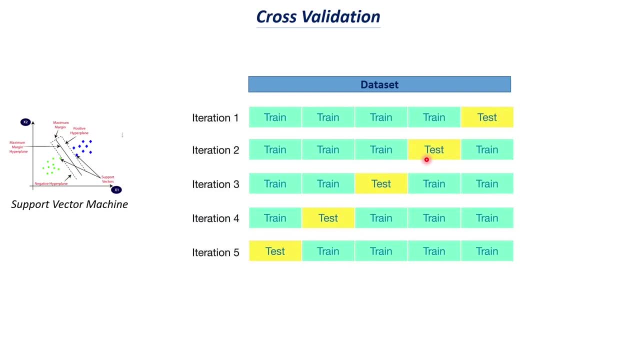 to discuss, which is cross validation. so let's say that we have two models- we have a support vector machine and logistic regression model, and we want to find which is which model is best suited for a particular project. so in that case we can use a process called as cross validation. okay, so you? 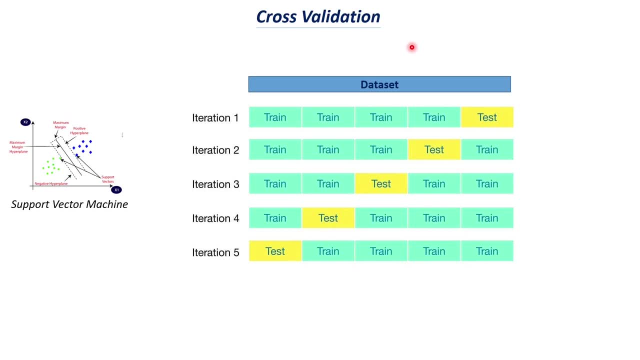 have this cross validation function in the library, called as sklearn as well in python. okay, so you can search as cross validation in sklearn. okay, so i'll explain you how this cross validation works. so first of all, we need to compare two models. one is support vector machine and the other one is 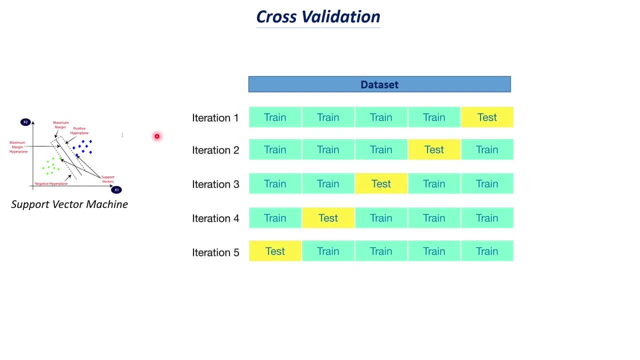 logistic regression. okay, so we try to find which model has the highest accuracy and, based on the accuracy of the model, we try to choose the best model for that particular project. okay, so let's say that that we have a data set. so let's say that we have a diabetes data set. so we have already. 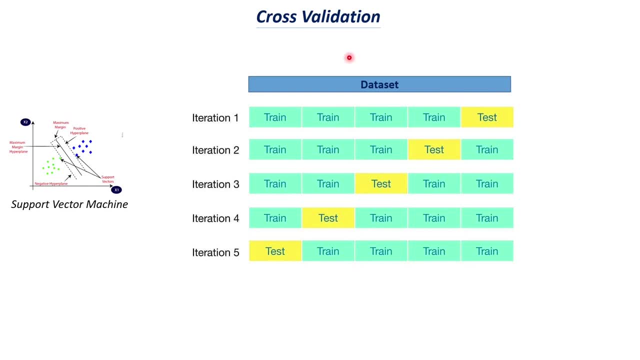 did a project on our channel on diabetes prediction. so this data set when we use cross validation. so what happens, is it? uh, so in this case we have about five iterations and this entire data set, so this complete data set is divided into five groups. okay, so we are just dividing the data set into five groups and the 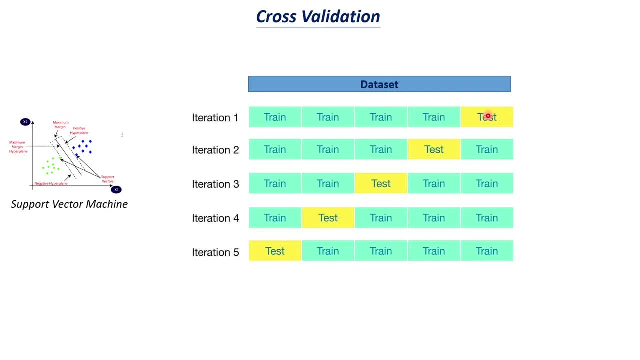 first four groups are considered as the training data and the fifth group is considered as the test data. okay, so in machine learning we split. we generally split the data into training data and testing data, and the machine learning model trains on the training data and the machine learning. 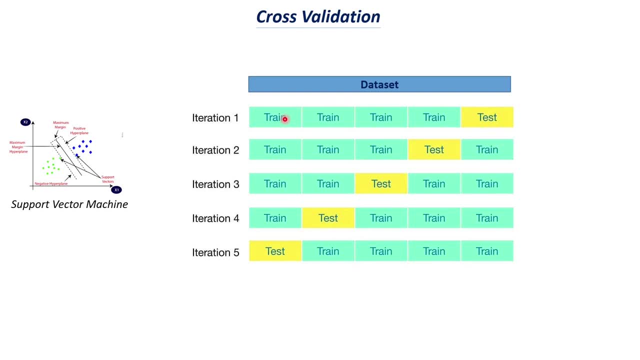 model is evaluated on the test data. okay, so in this case, we have four groups of training data and one group of test data and let us try to find the accuracy of the model. let us say that we have used all this training data. okay, so this four sets of training data to train our 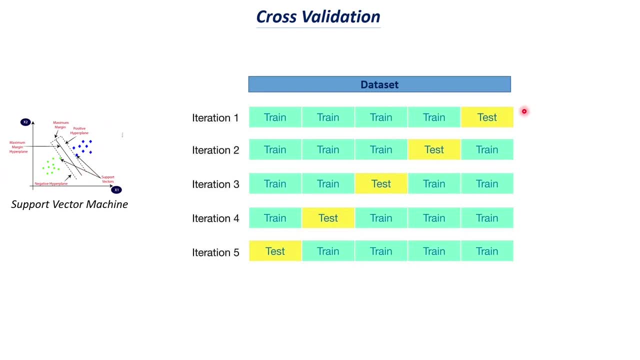 support vector machine model once it trains. we use this test data set to evaluate our model and we get accuracy score. so let us say that we get an accuracy score of 88 percentage. so 88 percentage means out of 100 predictions our model can predict correctly for 88. uh, you know problems, so that is. 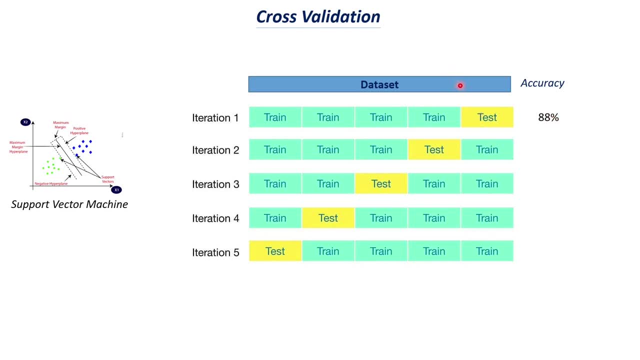 the accuracy represents. let's say that we are working on the diabetes data set, so we want to predict whether a person has diabetes or not. so when a model has 88 percentage accuracy, it means our model can predict for under out of 100 times. it can predict for 88 times correct value. okay. 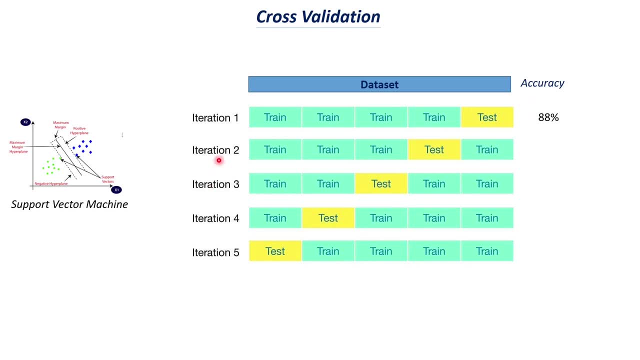 whether a person has diabetes or not. so, similarly, in the next iteration, what we will do is so we will again split our data set into five groups, and this time a different group will be considered as the test data set, and again we will- uh, you know- train the model. 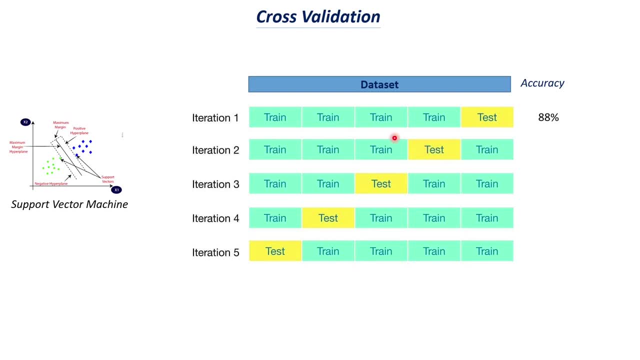 with uh, the training data and this test data will be used for evaluation and let's say that the accuracy we get is 83 in this case, and this process is repeated. so in the third iteration we have this particular third data set, as that is data in the remaining data test, uh training data, and let's say the accuracy is 86. and for the 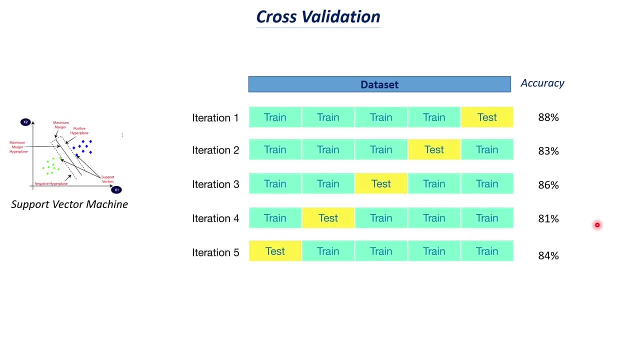 fourth iteration, the accuracy is 81 and the final iteration, the accuracy is 84. okay, so let's take the average of all these accuracies. so when we take the average, we get the accuracy as 84.4 percentage. so the reason we are doing it: we cannot, uh, just take one accuracy, so we need to. 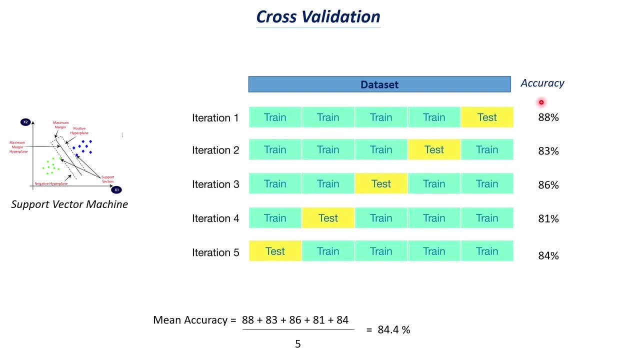 just have multiple accuracy to have a proper value or an accurate value. so that's the reason we are iterating it again and again. so this is the mean accuracy for support vector machine model. now what we will do is let's try to uh, do the same for the logistic regression model. as i have told you, we 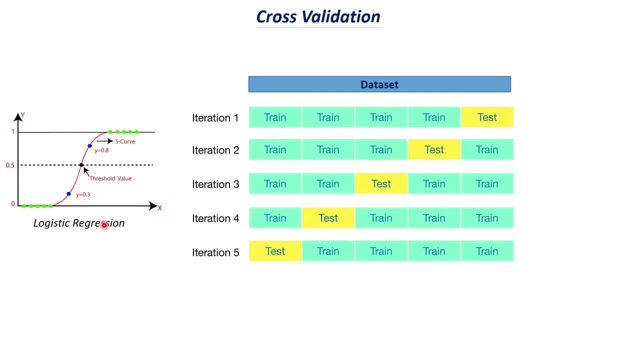 are comparing, uh, the accuracy scores of support vector machine and logistic regression. so we are going to- uh, you know, do the same thing again. so the only difference is we are using a logistic model in this case. so let's say that in the first iteration, the accuracy we get with the logistic 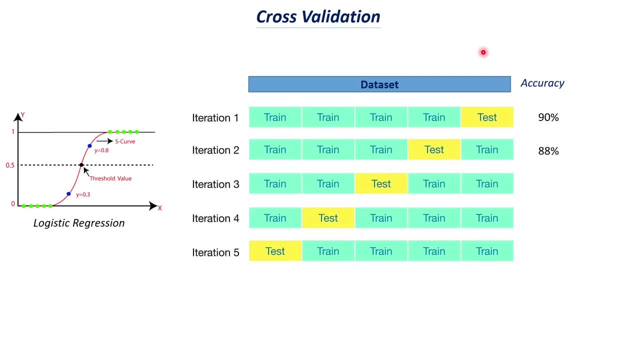 regression is, uh, 90 percentage, and for second iteration we get 88 percentage. and for third iteration, uh, the accuracy is 86 percentage, and for fourth iteration, let's say that the accuracy is maybe 91 percentage, and for fifth iteration, the accuracy is 85 percent. so this is just imaginary. 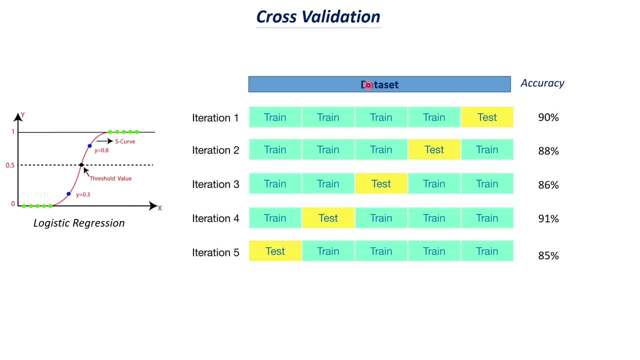 okay, so i'm just giving you an example. so this is, uh, the accuracy we get for this diabetes prediction. so, uh, in the first case, the for under values, the model can predict correctly about 90 values, and in the second iteration it can predict correctly for 88 values, and so on. 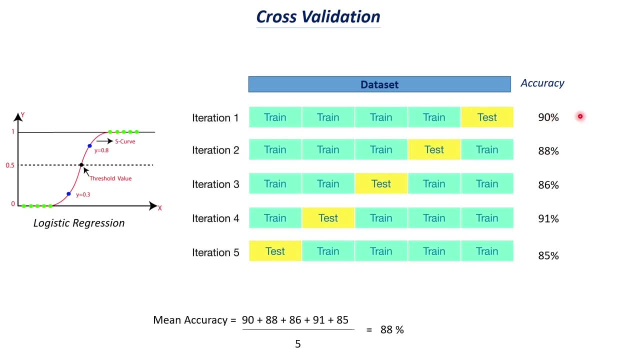 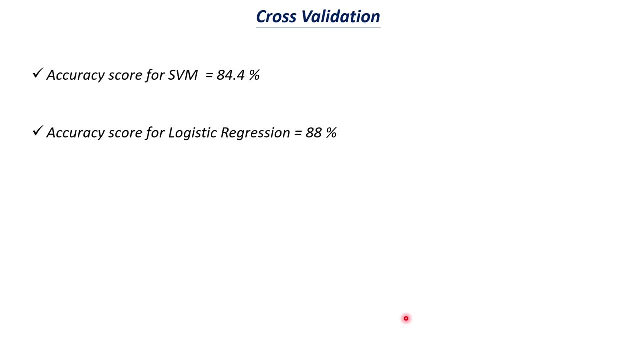 if you take the average accuracy for this particular logistic regression, the average accuracy, the mean accuracy here is 88 percentage. okay, now let's compare the accuracy of support vector machine and logistic regression model. so we found in this particular data set, the accuracy score for support vector machine model is 84.4 and the accuracy score for logistic regression is 88. 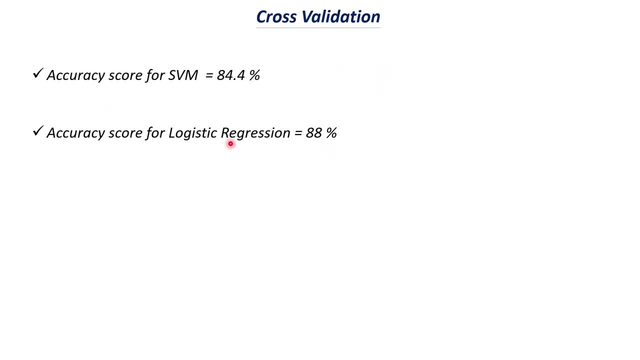 percentage. so, based on this accuracy, we can say that in this particular case, the logistic regression is the best model for this particular problem. okay, and this changes based on the data set we have. so we cannot get this particular result in all the cases, so it depends on the data set we have, on the task that we have and so on, as i have explained you before. okay, so 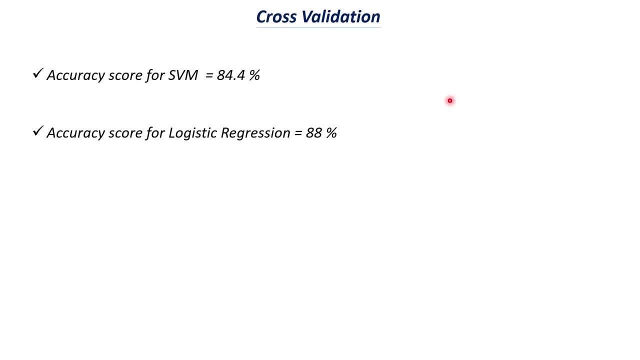 this is how you can compare two models based on their accuracy. i'll give you an example of how to implement this cross validation. okay, so you can just go to google and search cross validation or score in sklearn. okay, so it will take you to the sklearn documentation, where there will be this: 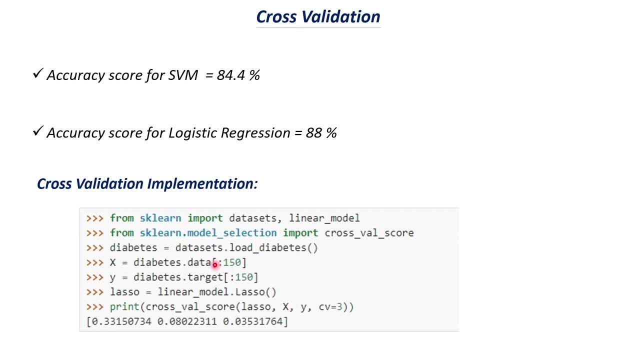 code snippet, so the official documentation of sklearn. there they have mentioned how to use this cross validation score. so in this, in this case, we are using this cross validation score to do the prediction on the diabetes data set. okay, so we are just loading the diabetes data set from here, from the sklearn, so you can see here. so from sklearn we are importing the data.